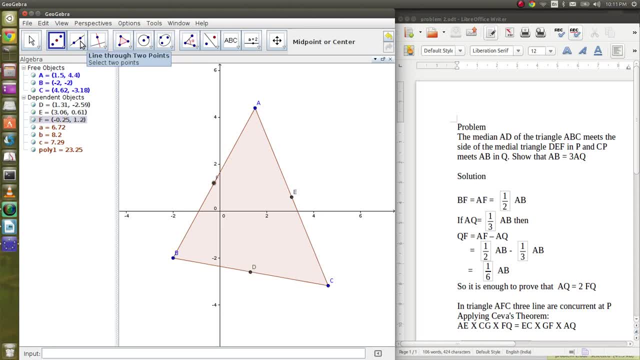 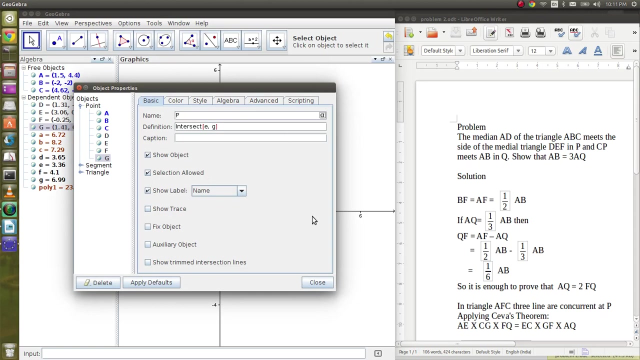 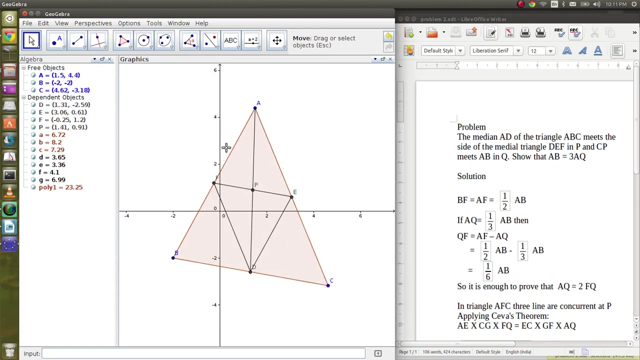 Now the medial triangle is made by joining. We are joining D, E and F. Let's do that. Now the median AD, We have to join the median AD. So this cuts the medial triangle in P, This is P, Okay, And now we have to join CP and extend it to AB. For that I use ray through two points: C and P. And now this is Q, And this point we name, it shall be Q. 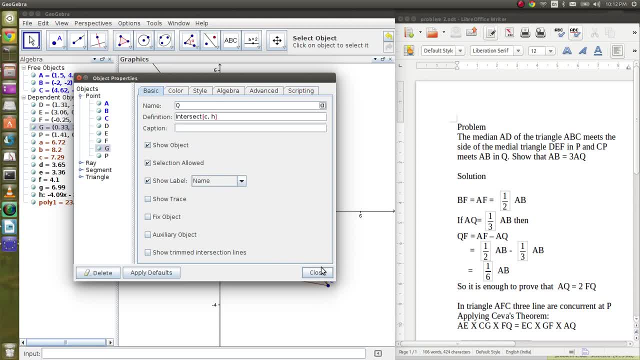 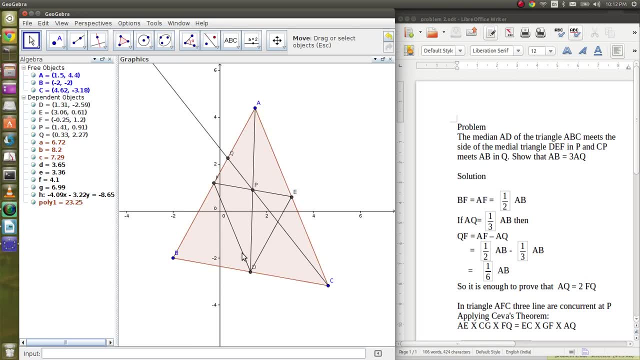 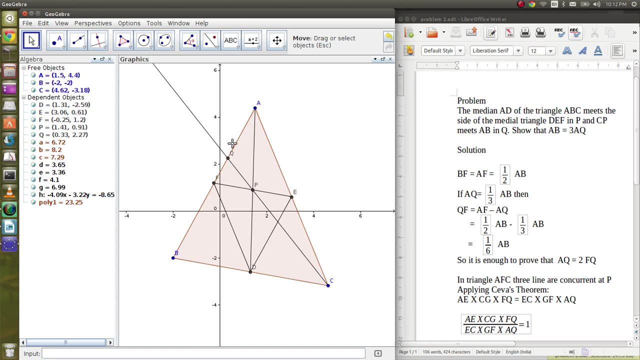 Now we have to prove that AB is equal to 3AQ. As we know, BF equals to AF. F is the midpoint Equals to half AB. Now in AF, if AQ equals to one third AB, then QF must be half minus one third. one sixth AB. 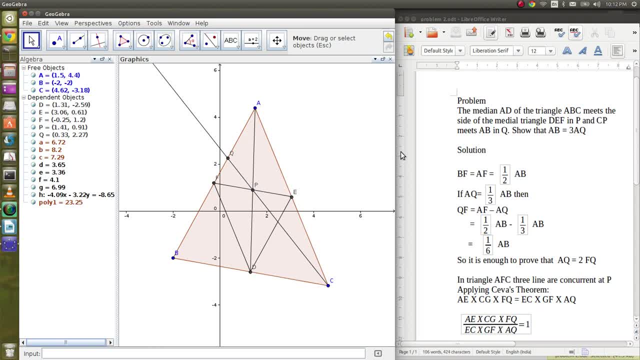 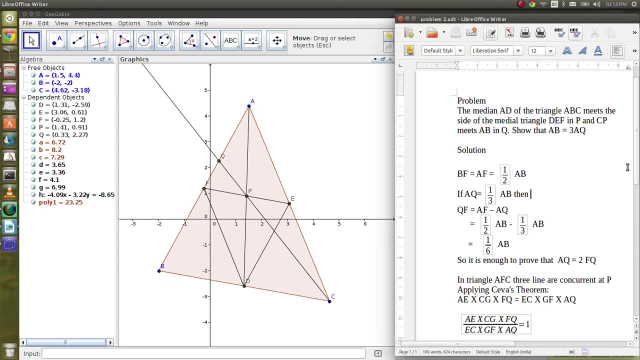 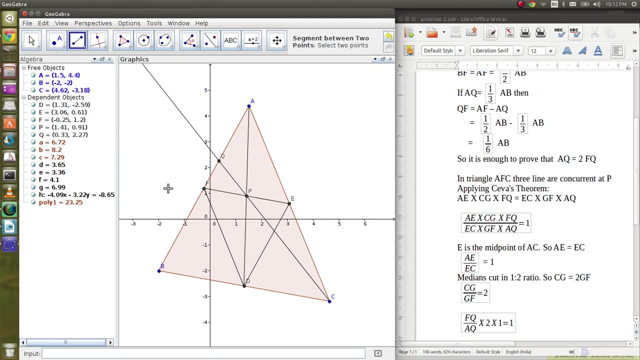 QF is half of AQ, So it suffices to prove that AQ is double of QF, This one. So we join F and C Again. this is a medial- And name this point G. Okay, Now consider triangle AFC. Here we find that three concurrent lines meet at the point P. 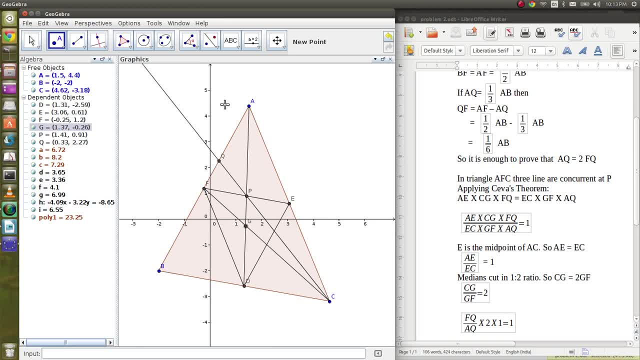 So we can apply the Siva's theorem, Which is AE into CG, into FQ, equals to EC- into GF, into QA, Which leads to AE into CG, into FQ, by EC into GF, into AQ, equals to one. Since E is the midpoint of AC, AE by EC equals to one.